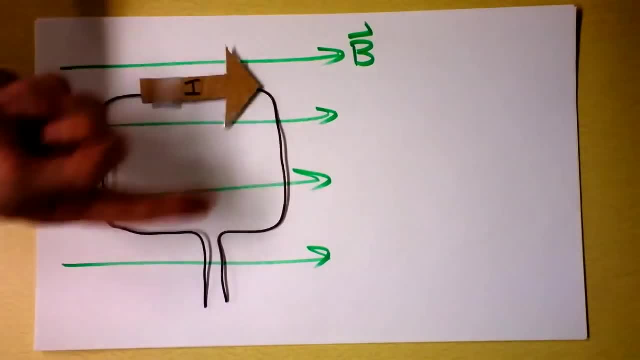 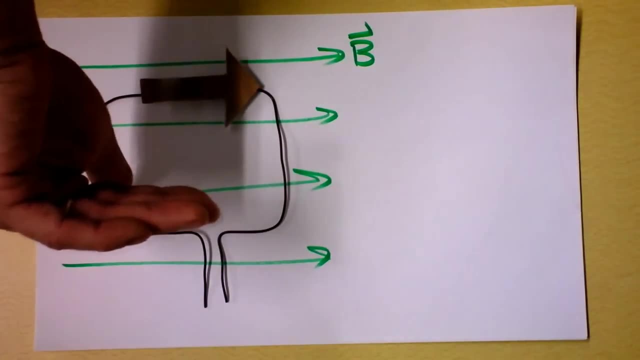 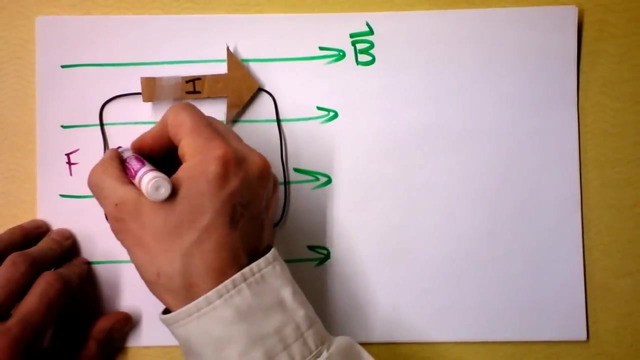 but they're going this way and the magnetic field is that direction. so I'm going to put my like that and then go like this, and I see that my thumb is pointing into your screen and into my page right there. So there's a force that's inward over here and I draw 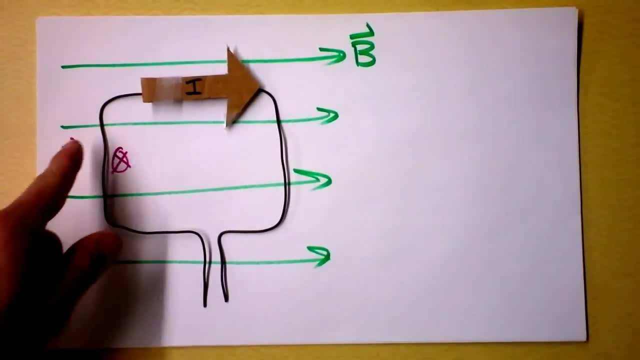 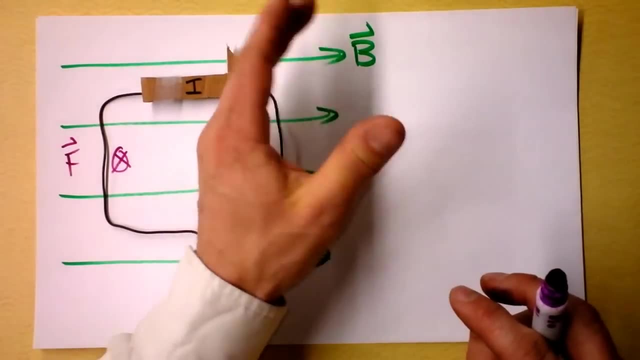 it like that. That's the direction of the magnetic force on this current carrying wire, And there are also electrons. Let's continue. the electrons- They're going this direction- and magnetic fields that way. If I do that, then you see that the force is outward in this case. So there we've got. 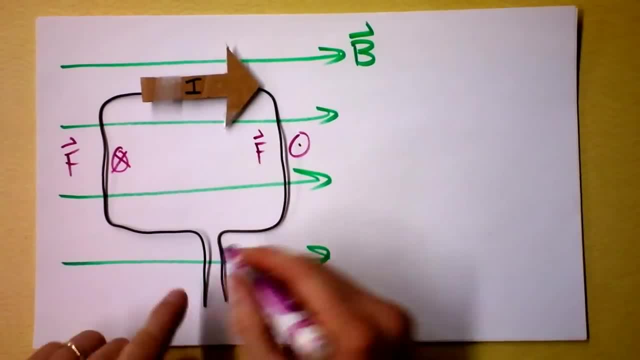 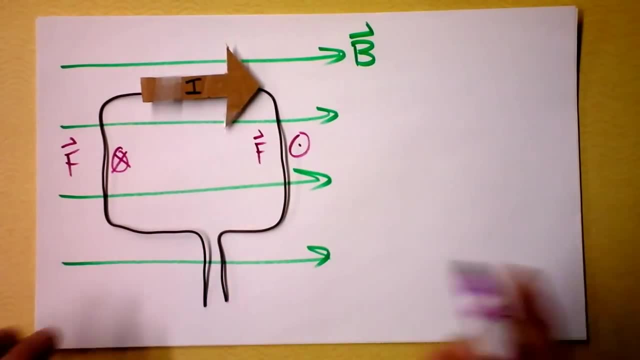 an inward force and here we've got an outward force and there's no force on the top or on the bottom and there's some force on these guys, but it cancels out and they're kind of right in the middle and right next to each other and we try to make sure that there's. 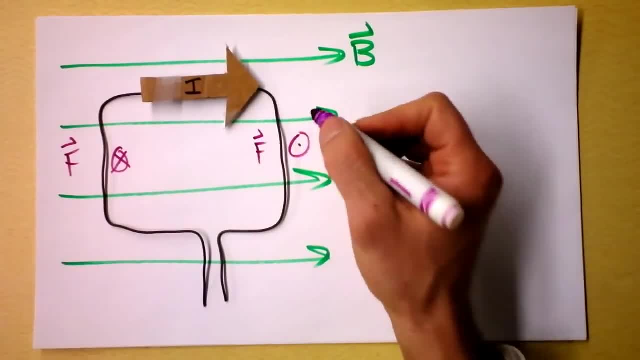 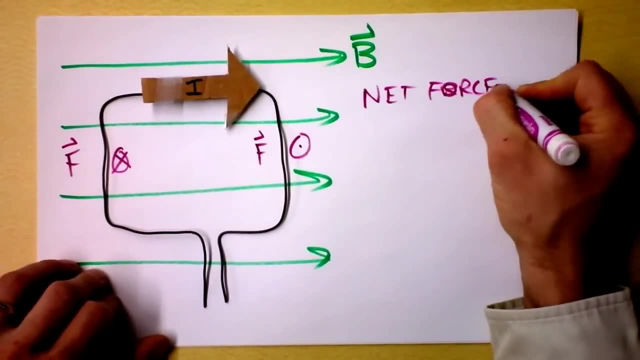 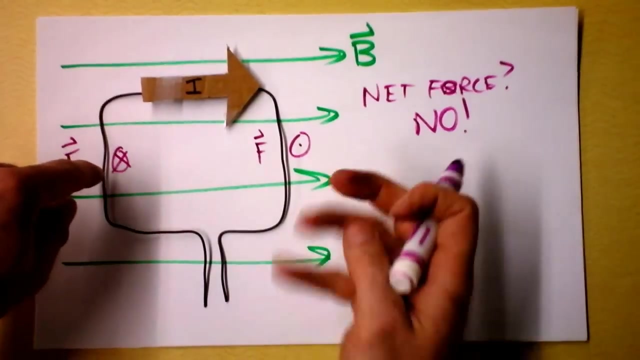 only this force here and that force there. That force, wow, is there a net force? Oh, my gosh, Oh gosh. Is it doing anything at all? then If I push that down and I pull that up at the same time, we're going to get a net torque. Okay. 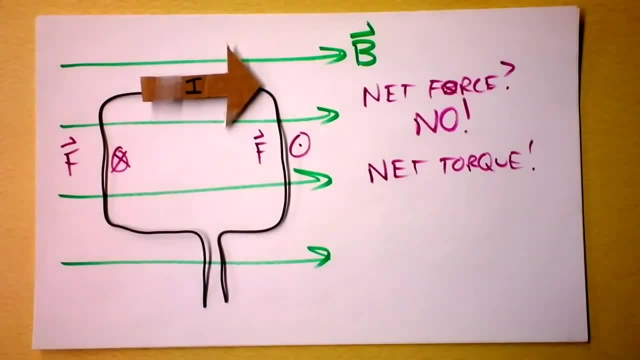 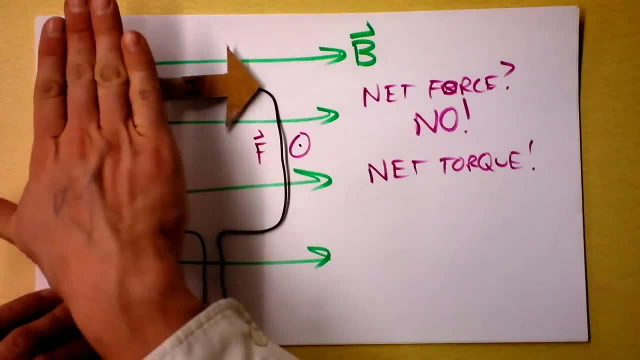 That's pretty exciting. Now let's look at it again from the perspective of the current though. Now we pretend that there are positive charges moving this way. so I'm going to say positive charges that way: magnetic field. I'm using my right hand. 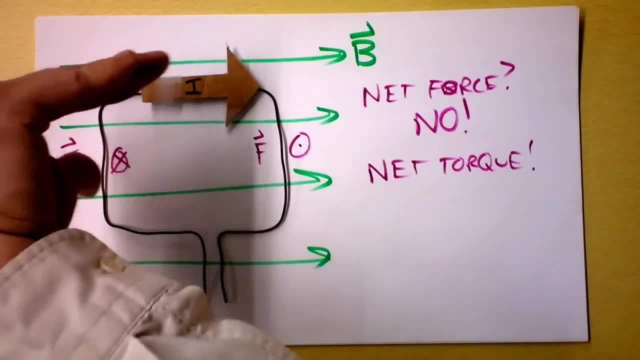 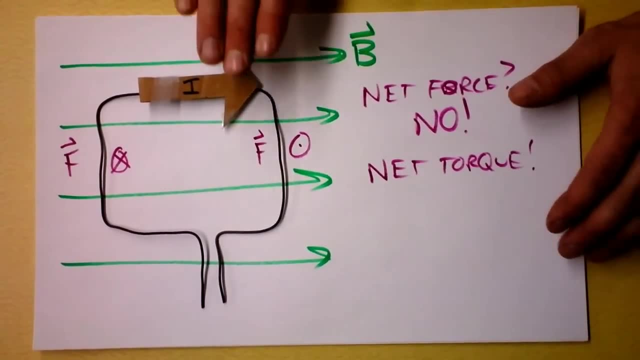 this time magnetic field, that direction. So I go like that and I find that the force is still into the page. And if the magnetic field is to the right and the current is going down, then I go like this and I find that the force is out of the page. 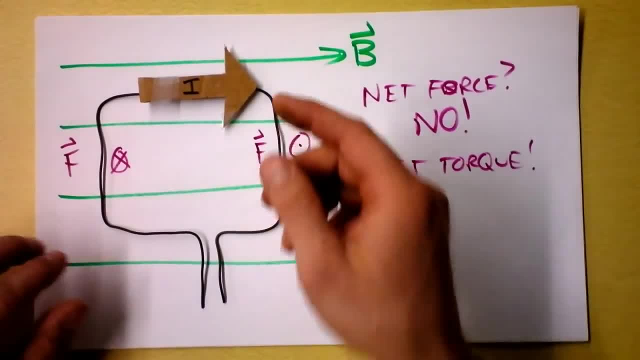 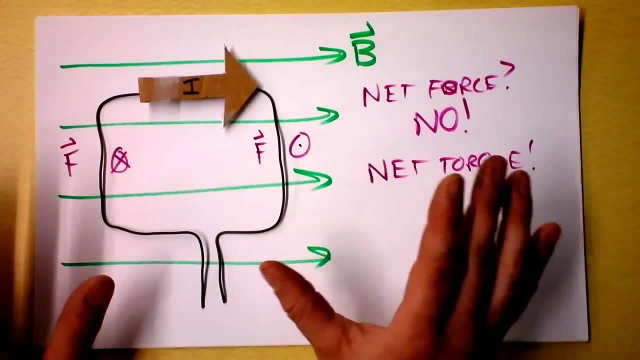 So I don't care whether you say electrons are going this direction or protons are going that direction. you're going to get the same direction for the force. So whether you're honest about it or you just gloss over the whole effect that Benjamin Franklin got the current wrong, it doesn't matter. 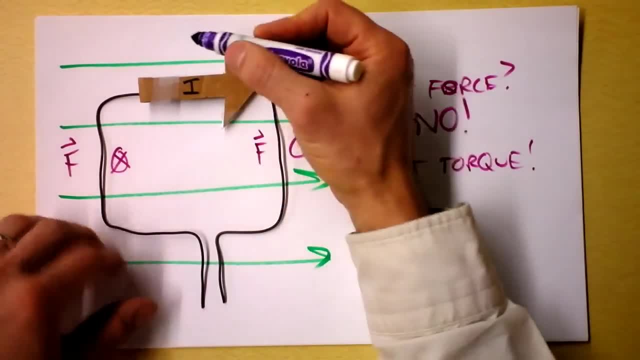 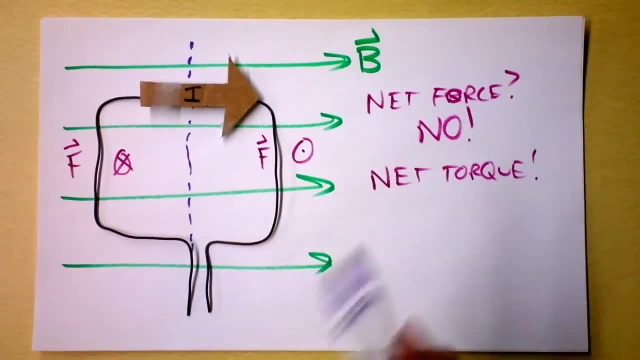 You're ready to rock? There will be a net torque on this sucker and it will rotate about this axis. So I'm going to put an axis right here that it can rotate about, and we want to figure out how much that torque is. 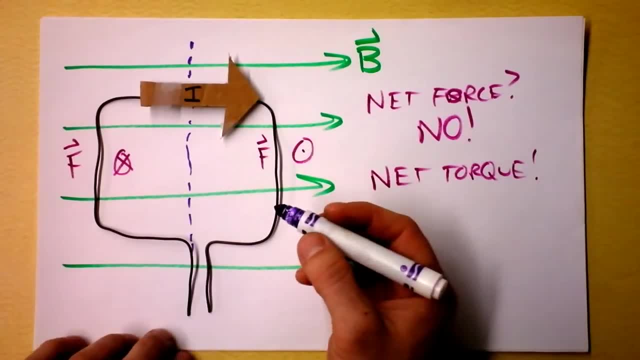 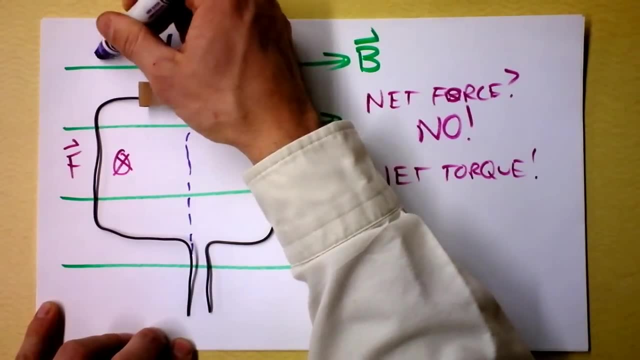 So I have to define some quantities here. I'm going to define for you the width of my loop, That's a W, and it'll be from there to there, And I'm also going to define the H. Now, the H, this is the height of my loop. 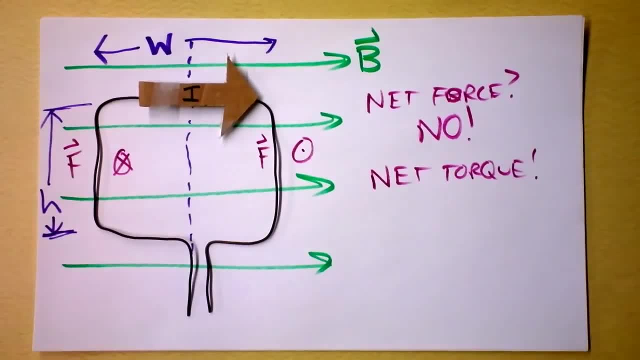 H is the length of the loop And this is the wire that's feeling the force. So that's going to go into my BIL equation, But we're using the H because it looks like a height right now. So I know an equation for torque. 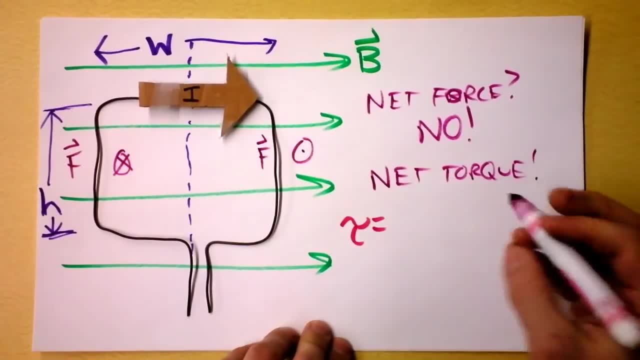 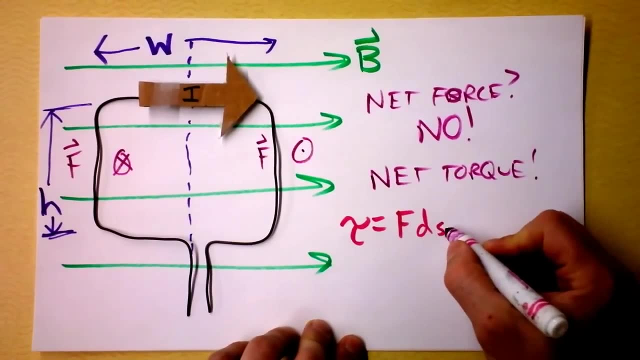 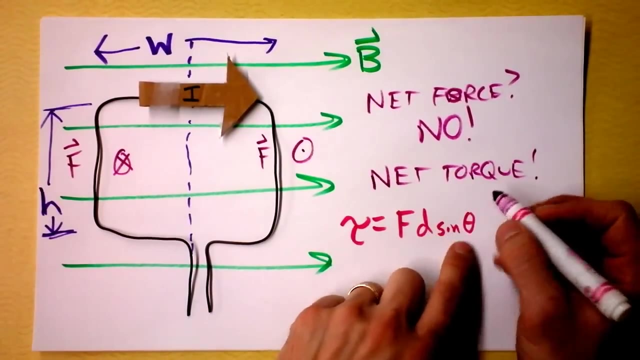 and the equation for torque is this: Torque is well, it's got to be force times, distance times, the sine of the angle between the force and the distance right. And in this case I'm going to find well, guess what. 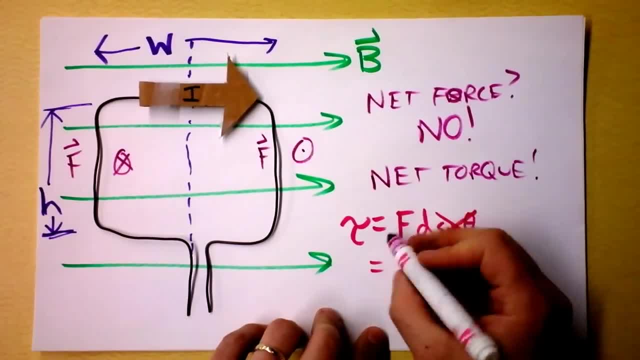 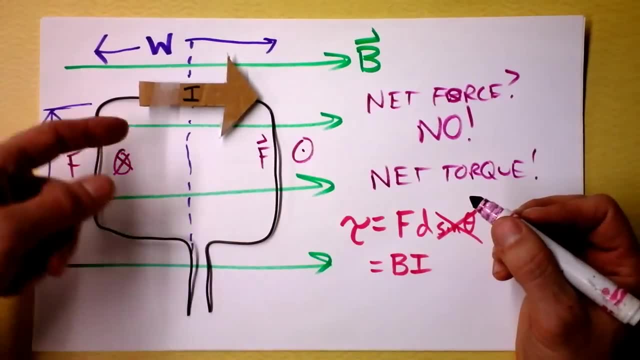 We've already taken care of the sine, so that's fine right there. The force is BIL, right, Which is B times I, magnetic field strength, times current strength and I guess more force, more torque, rather, if the field's bigger. 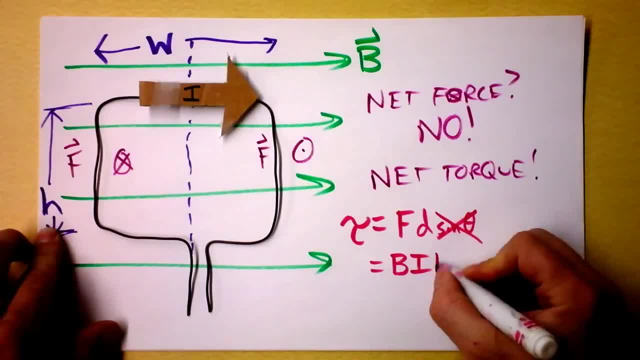 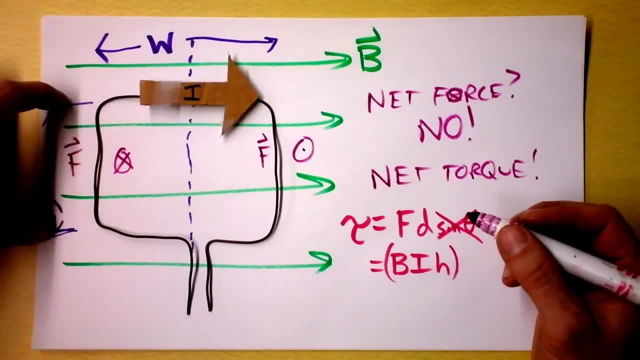 and more torque if the current's bigger, sure. And then I have to multiply this by H, because H is the length of the wire. that's feeling the force. It's not feeling a force until it turns, and there it's feeling a force. 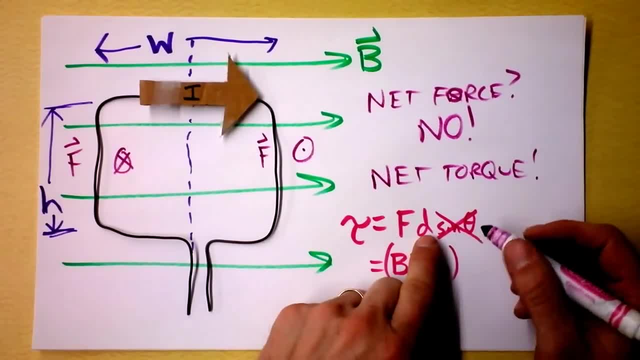 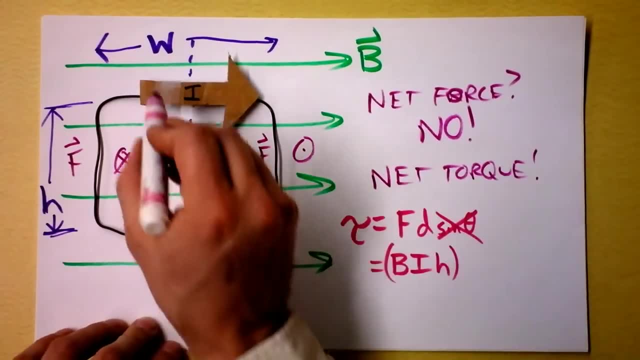 And it's not feeling a force after it turns up there. So I'm going to then multiply that by the distance. what is this? D for a torque? Oh shoot, That's distance away from the axis of rotation. So in that case that's going to be half of W. 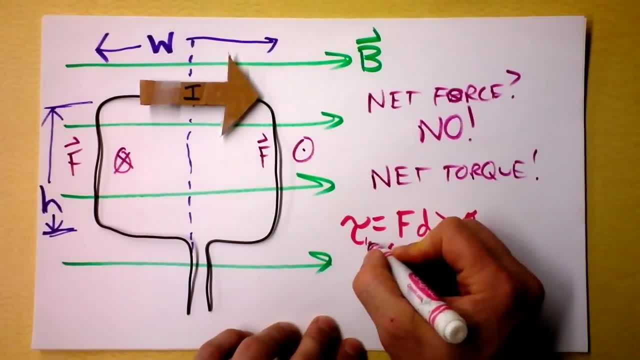 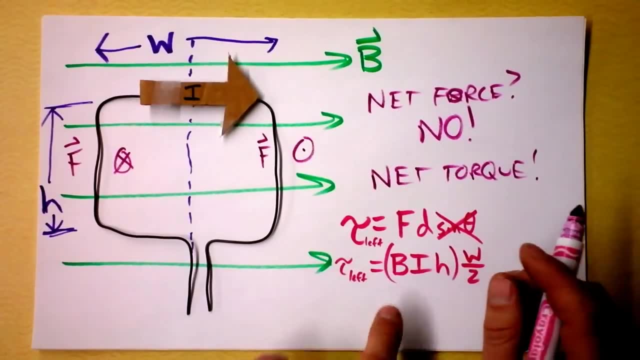 So I say W over 2.. This is I'm going to say. this is the torque from the left side. Torque from the left side is that big right there- And torque from the right side. wait a second, is this positive or negative? 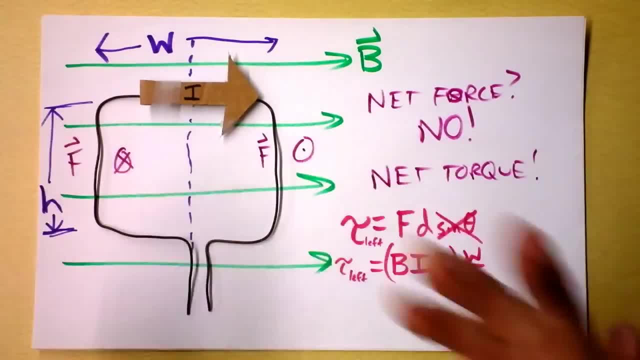 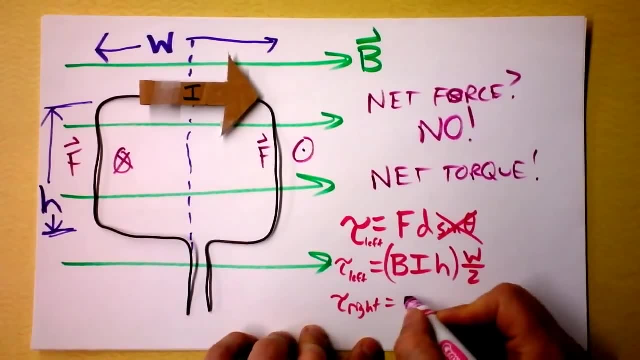 It's going to cause it to rotate that direction Like that, And so I don't have to worry about whether it's positive or negative. But look that torque from the right is exactly the same quantity. It's B times I times H times W over 2.. 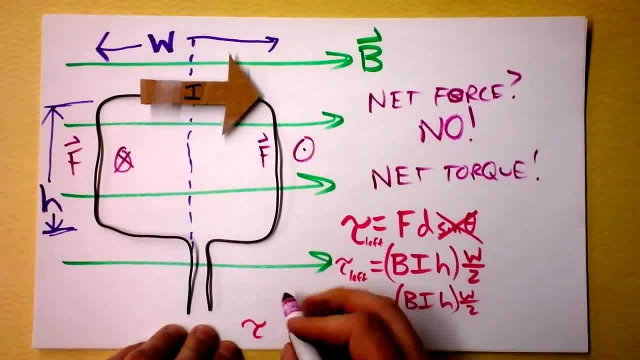 And then I can say that the torque on the system, the torque on the system is just the current times. the times, well, it's going to be current times. I'm sorry, I'm totally looking at this the wrong way. 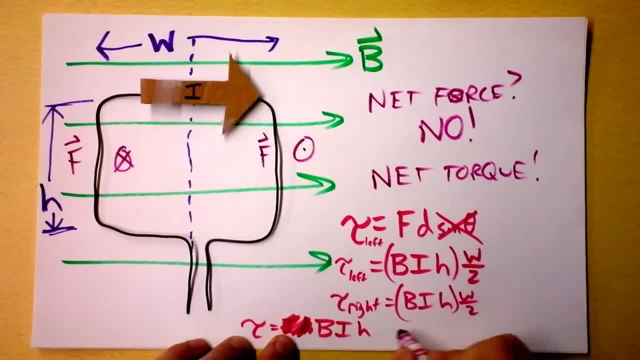 It's magnetic field times, current times, height times, width. If you look at that and it says height times width, that's height times width. what is that for that loop? That is in fact the area, So it is. then we can see it as B times. I times the area of the loop. 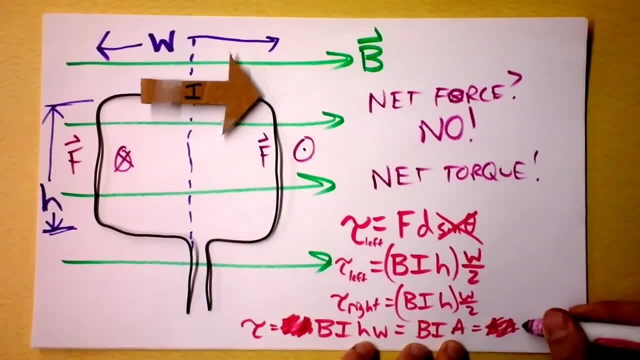 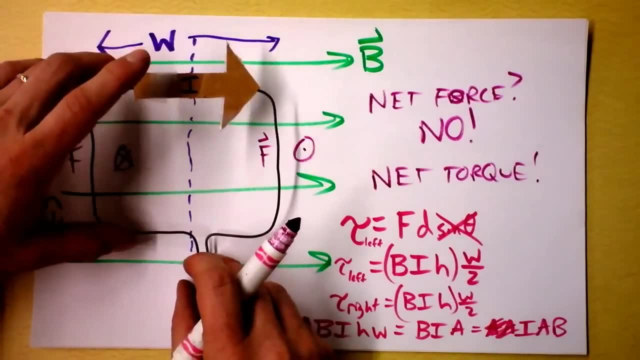 And it's usually written as I wow, I times A, times B, And that's only if it's in a favorable orientation. I guess, if I had it at some other orientation, like this, as it's gradually going, as it's gradually going to here, 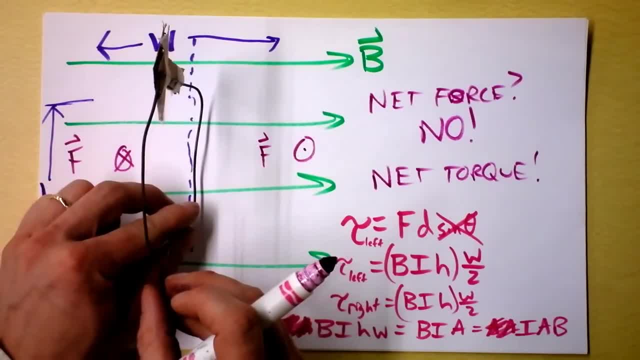 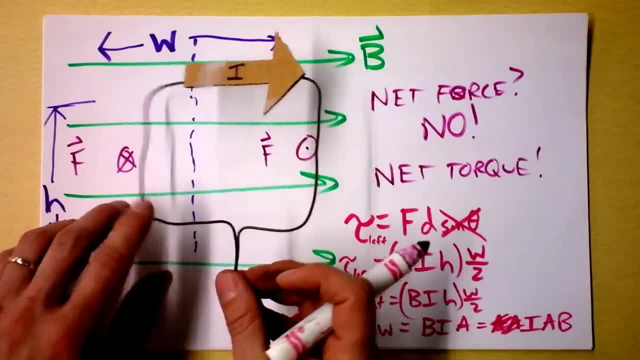 that will be. wait a second. it's going to go like this As it's getting to this orientation: right here there's actually no torque at all. So let's think about this: Big torque, no torque, And we'll do a top view so that you can visualize that. 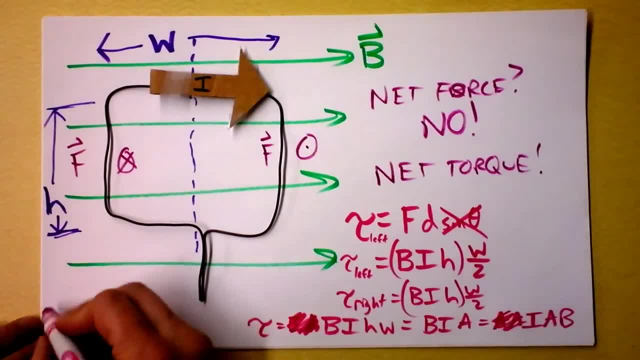 But we're going from big torque to no torque, so we have to in fact add a little bit of a sine of theta. Torque is I times A times B times the sine of the angle between- ooh, remember this area vector. 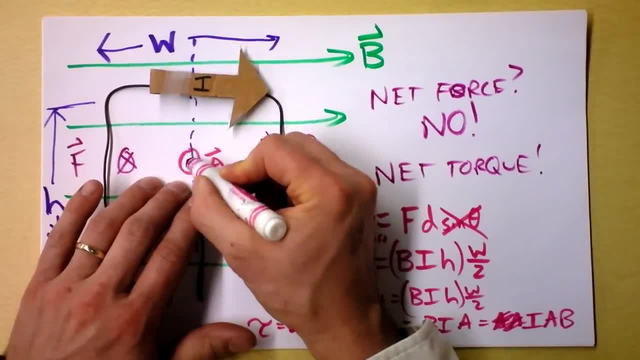 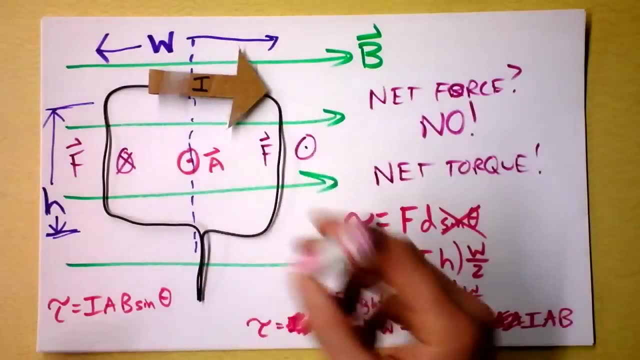 The area vector points out. The area vector points out right in the middle, And so right now I've got a big torque because the area vector is pointing straight up and the magnetic field is pointing directly that direction. so I've got a very big torque. 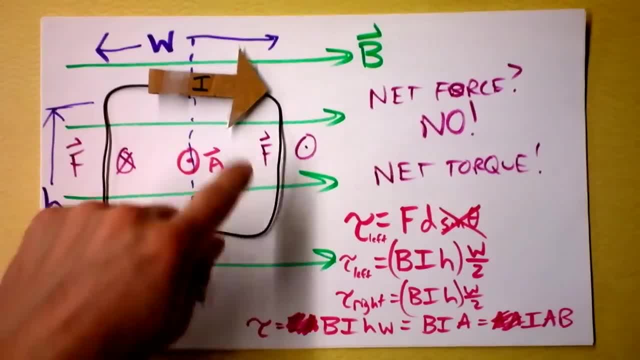 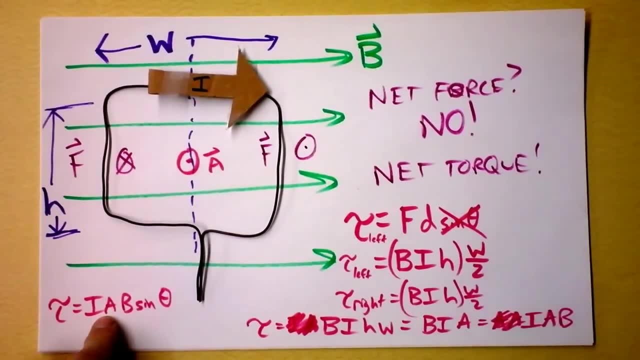 And I want to say first that this, which we derived for a rectangle with height and width, generalizes for any area. We can in fact, always use A, And that's, that's awesome. So then I want you to say: 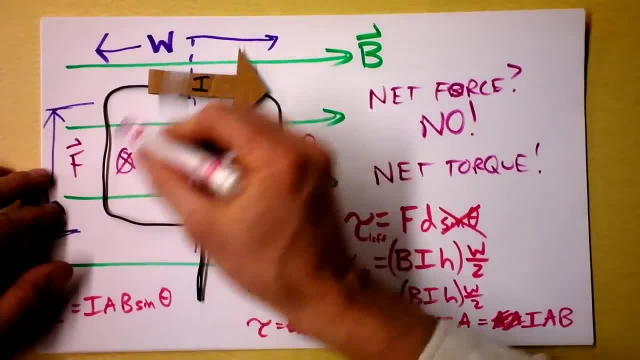 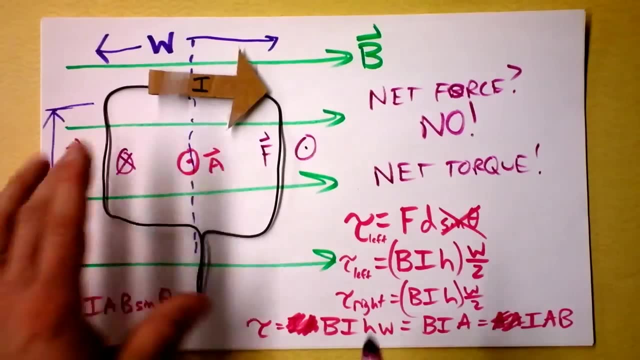 should we do a top view first? No, let's continue this. If, what if I had more loops, If I had a loop going this way and then, instead of leaving the loop, I just went: another loop, two loops, or three loops, or four loops. 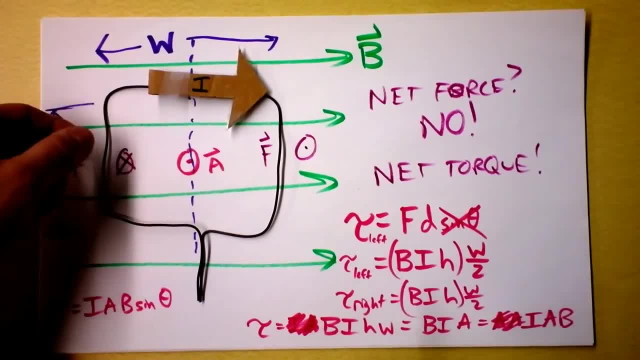 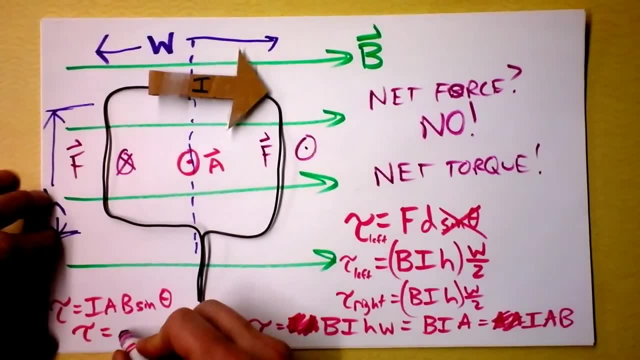 you can imagine that this force would get bigger and bigger and bigger, because it's effectively more and more current here and more and more current there as I'm adding more and more loops of my wire. So then I can get to this equation: Torque is the number of loops. 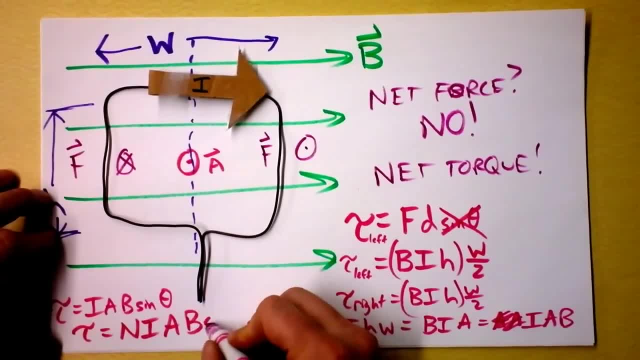 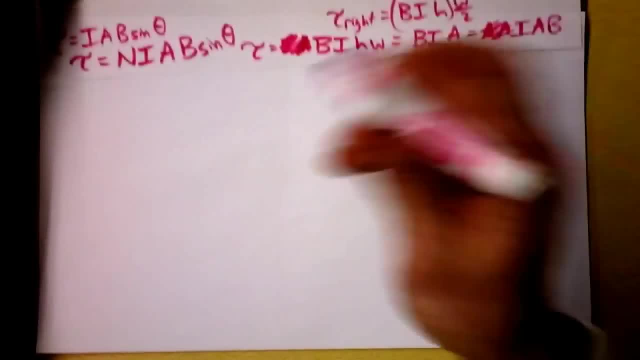 times the current times, the area times, the magnetic field times the sine of the angle between them. We're going to write that equation on the next page and then say something cool about it, and then we'll do a top view. The torque of a current-carrying loop. 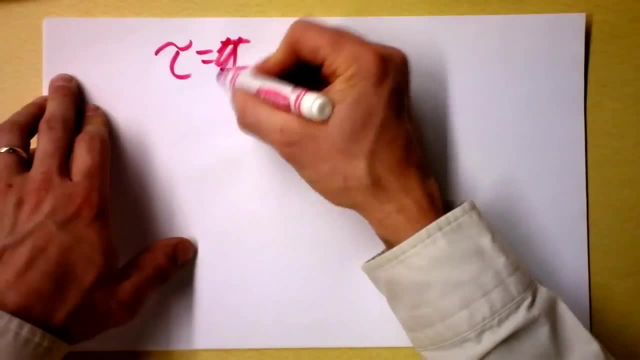 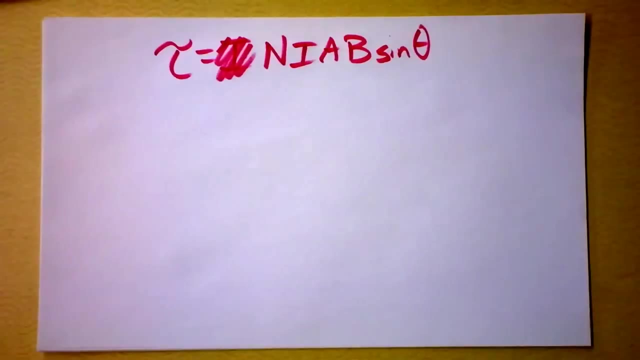 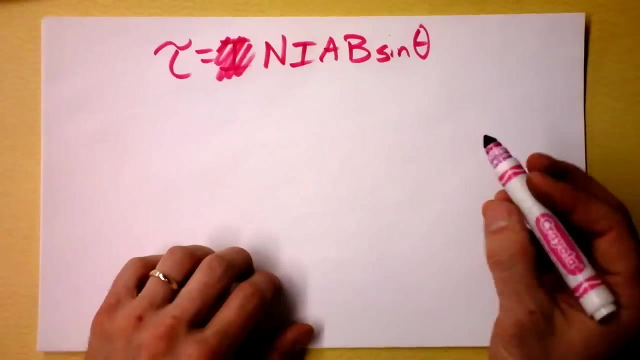 the torque that the current-carrying loop feels when it's in a magnetic field is dang it N times. I times A times. magnetic field times the sine of theta. Oftentimes you might want to separate the geometric, the geometric contribution. 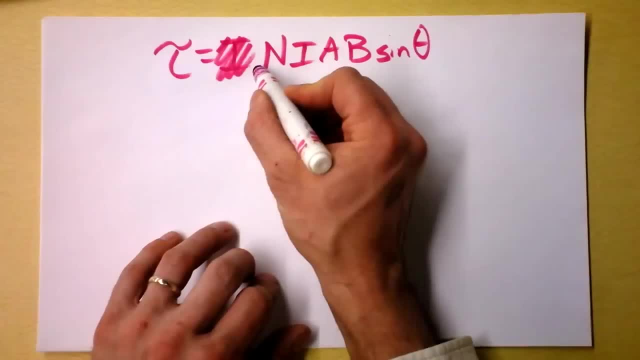 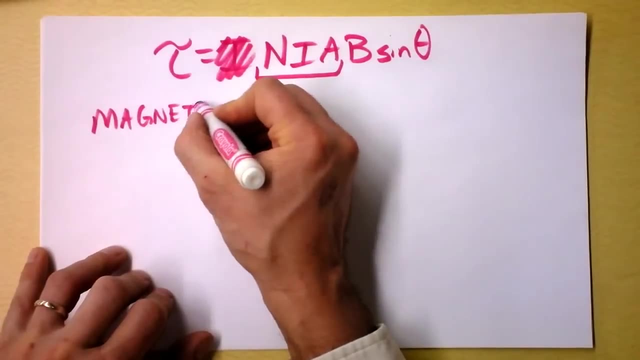 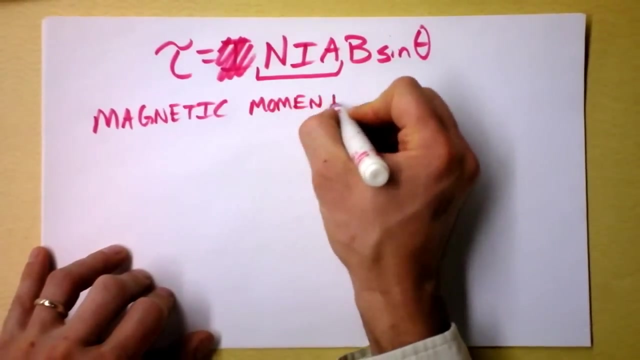 from the external contribution. So this part right here is sometimes called the magnetic moment, And because that came up a little bit in a book that I wrote, you might want to study the magnetic moment as a separate thing. It will help you as you continue your study of physics. 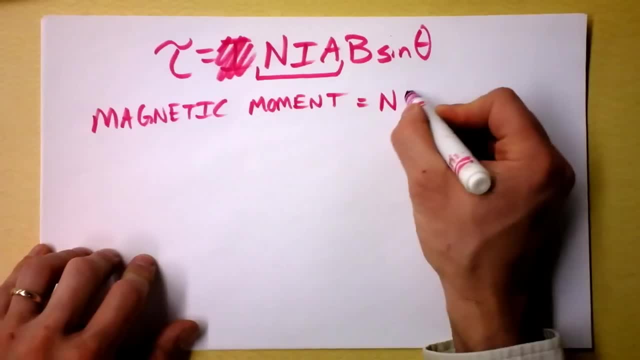 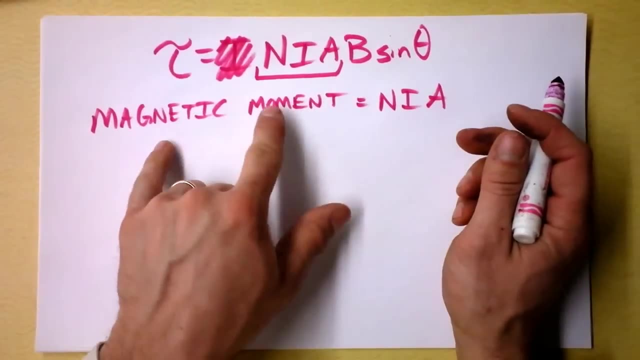 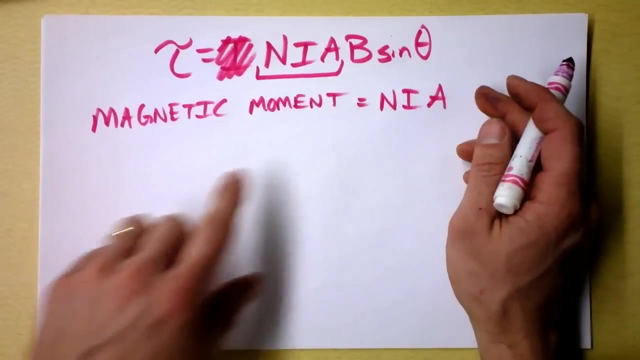 Magnetic moment is N times I times A. So what I'm thinking is torque on anything is the magnetic moment times the magnetic field and with an orientation correction right there. But the magnetic moment depends on how many loops you got, how much current you got going through them. 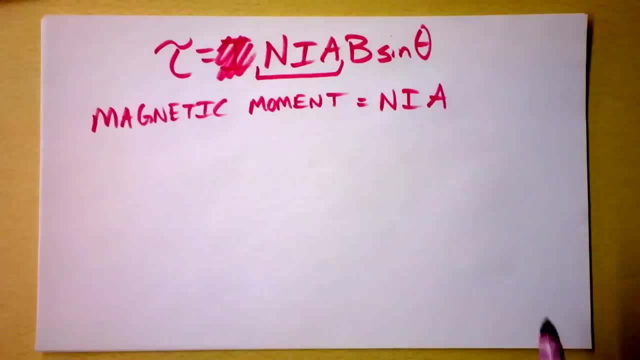 and how big that loop is. So the bigger the loop you get yourself a loop like this, that's not much torque. You get yourself a loop like that, that's a lot of torque. So we can change the amount of torque that we've got. 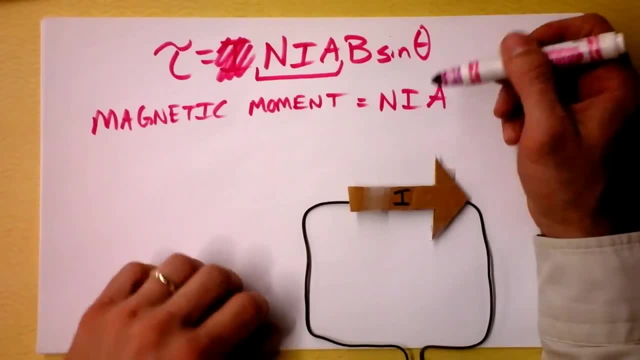 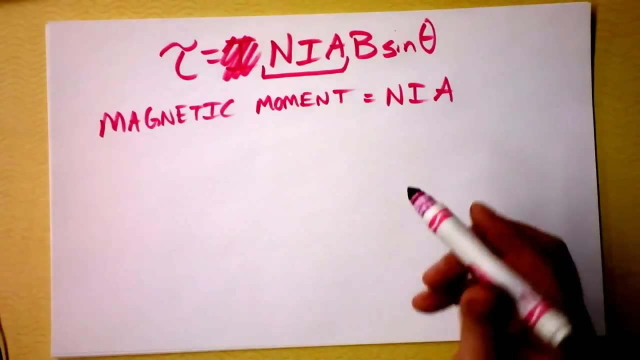 based on the well, based on these three factors and the external magnetic field, which we presume might be out of your control, But maybe it's in your control too. Alright, it's time for a top view, And in the top view I get my magnetic field. 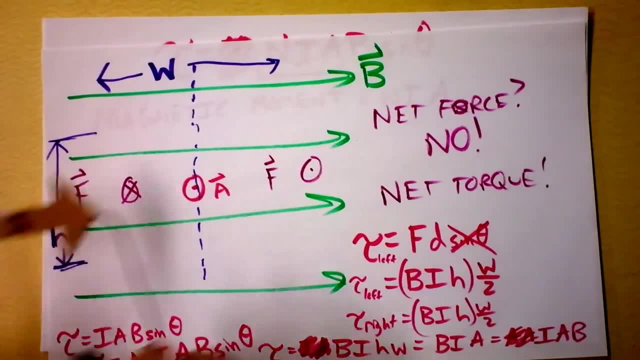 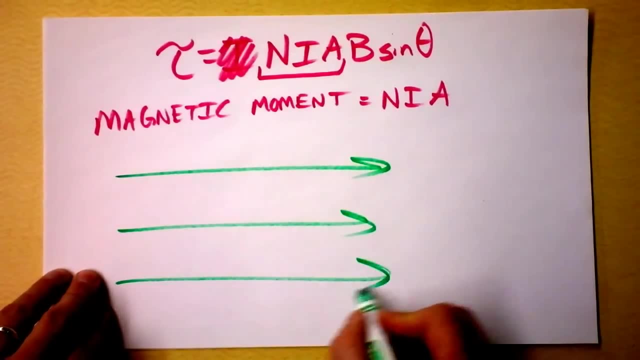 and it's still going to be. we're taking this picture right here and I'm going to draw a top view of it. So I've got a magnetic field pointing this direction and, initially, my orientation of my loop. what was I saying? it was going to be a top view like this: 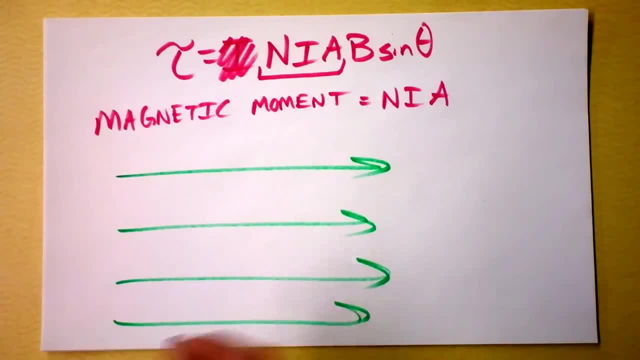 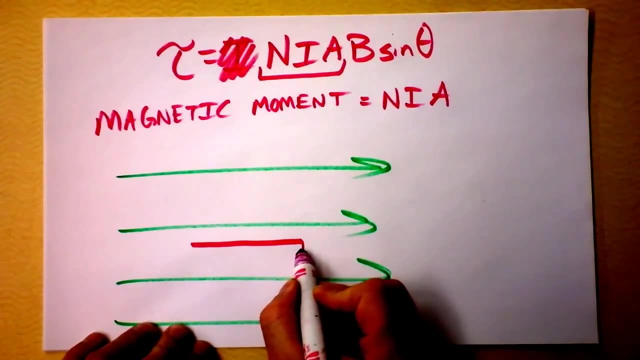 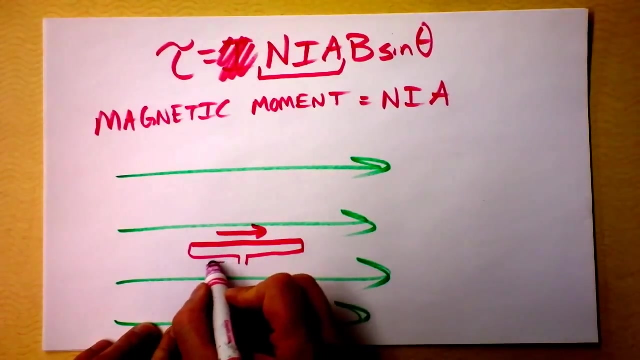 My orientation of my loop is like: well, it's like this. It's standing up here because it's a top view And I've got current going in my loop this way. Current is that way And then here it's that way. 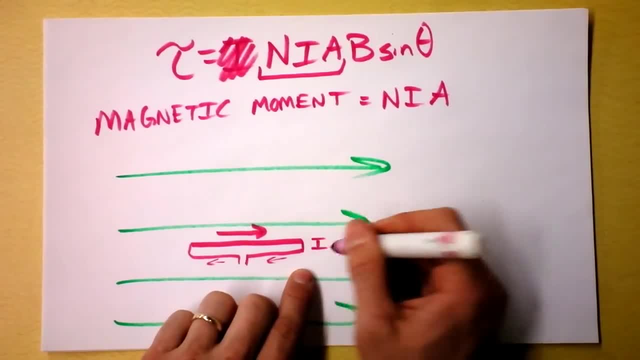 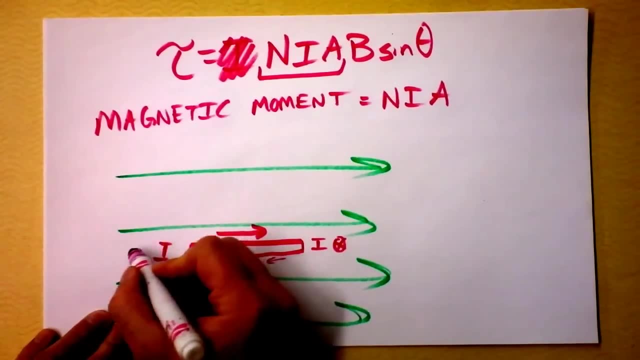 and there it's that way. So this current right here, that current is going down into my page and the current over here is going, oh, gosh up out of my page And notice that the current on the top and the current on the bottom, 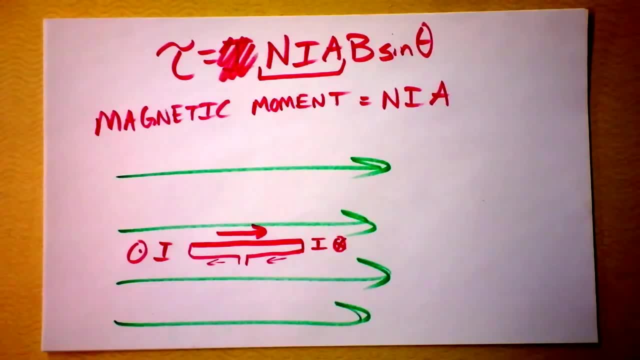 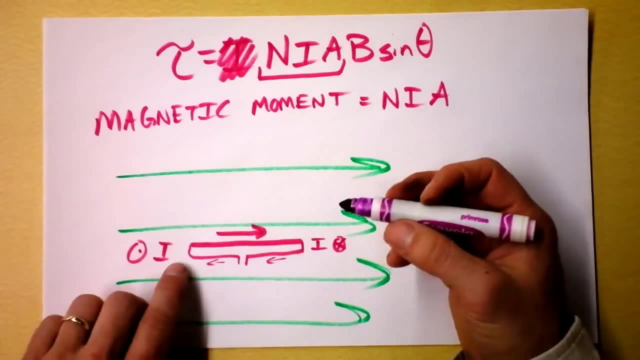 don't have any forces. So I get forces. I'm going to draw my forces. I'm going to draw my forces in primrose or something I don't know. Yeah, primrose, All right. So I've got a velocity of positive charges out of the page. 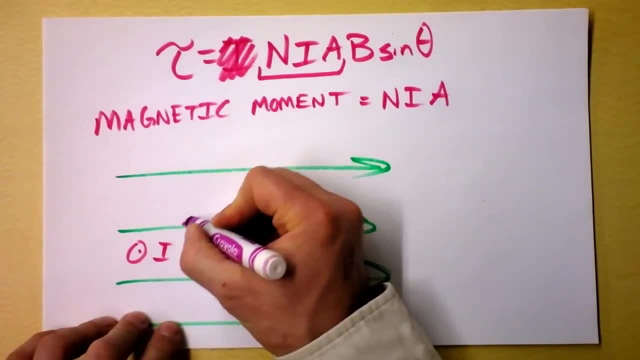 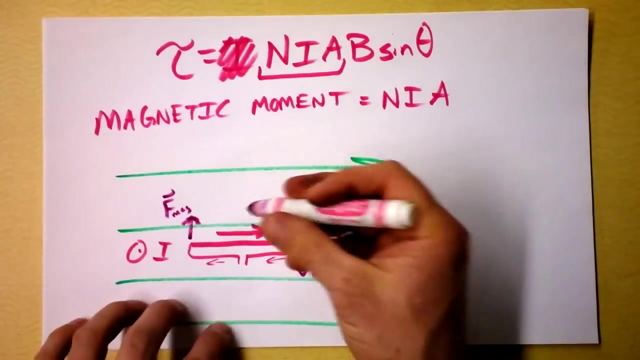 and a magnetic field that direction. So the force here is that way and the force here is that direction. That's the magnetic force on those current carrying wires. But as I move to this orientation it will gradually spin to this orientation. I'm going to say that it will be in this orientation. 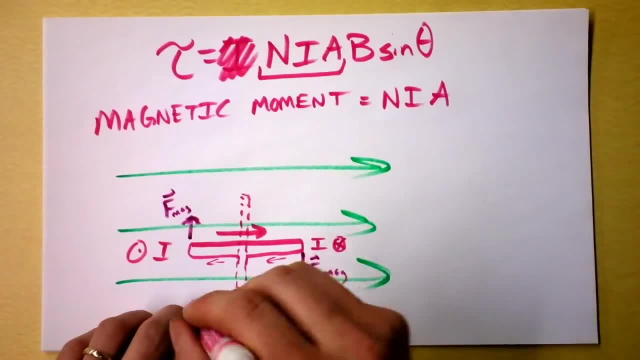 in a little bit And still I've got current. that's down and down and magnetic field- Oh shoot, Magnetic field is still that direction, because I just did a top view And well, let's figure out what's going on here. 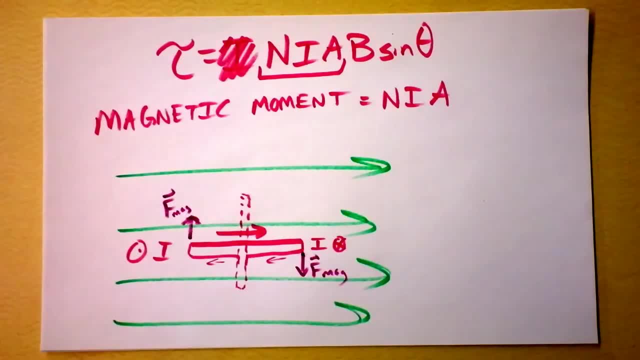 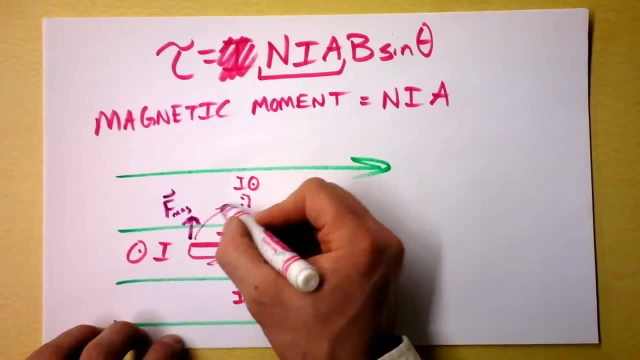 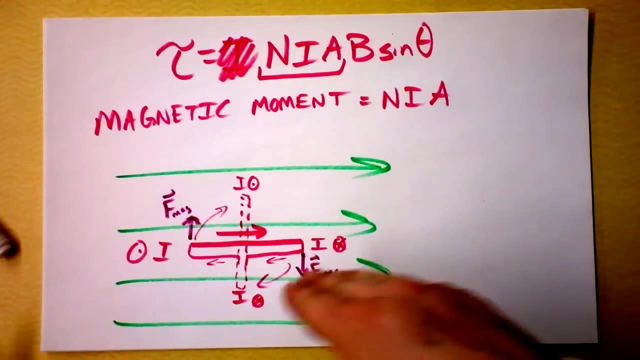 At this instant I've got current that's going down. So I should note that I'll have current into the page and current out of the page right here, because I simply rotated the whole thing to that orientation because of the torque And if the current's down into the page. 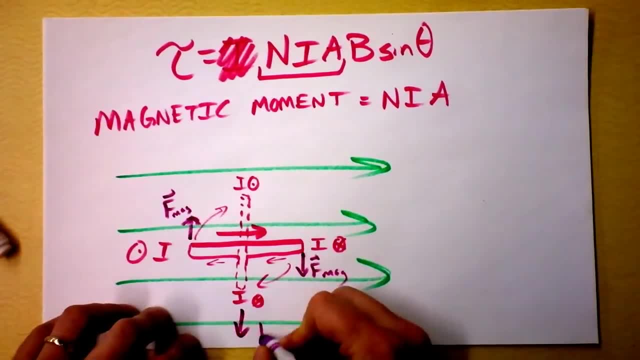 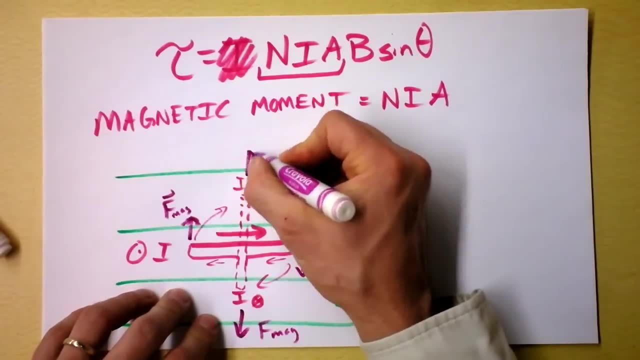 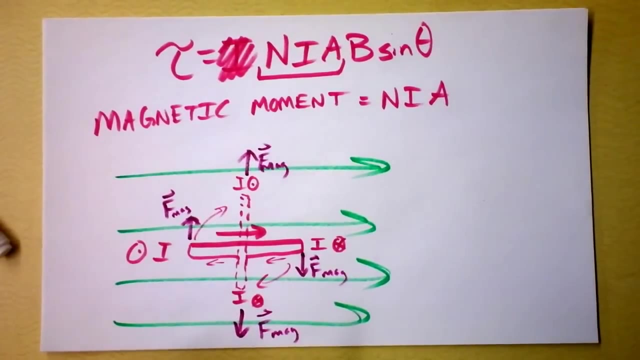 and the magnetic field's that way, then the force is simply out. And if this current is up and the magnetic field's that direction, then this force is also out. That's my magnetic force there and my magnetic force there. That's not a torque at all. 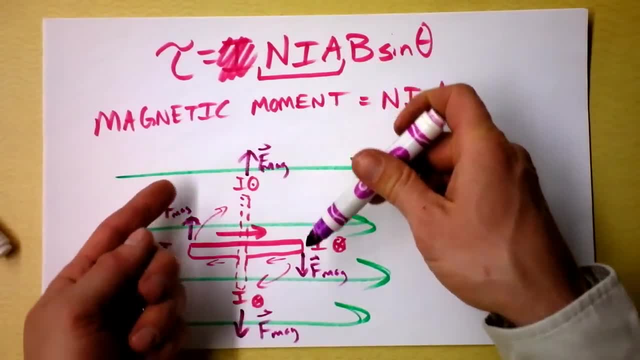 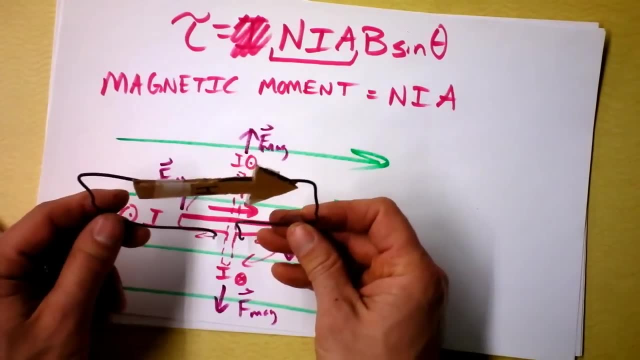 But guess what The cool thing is, this will continue spinning because it's got inertia, It's got rotational inertia, It's going to continue spinning. I'll set it up like this: I've got current going that way and it's going to continue spinning. 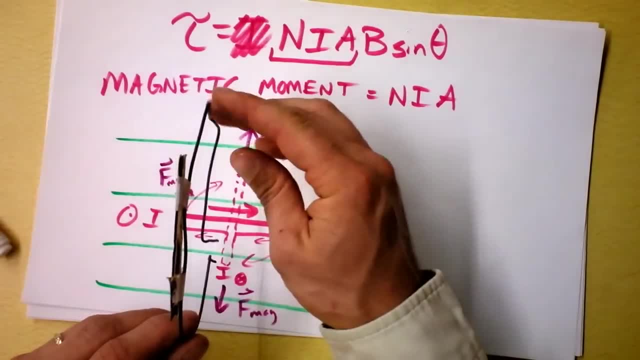 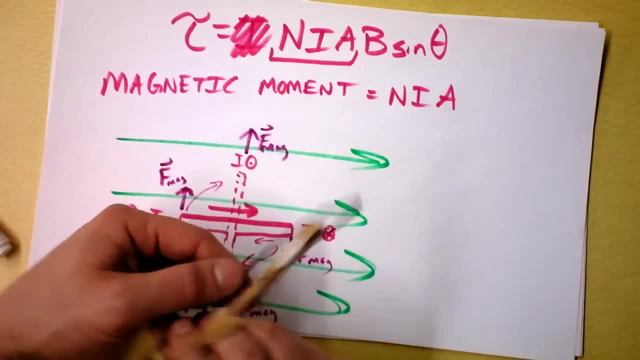 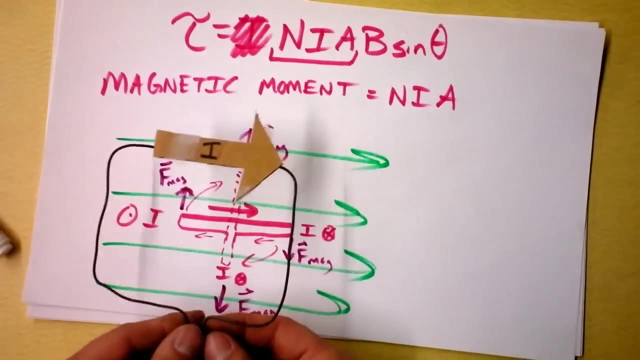 It'll have here a whole bunch of speed And eventually it gets a torque the other direction. So it will go back this way and you can see that it will go. What if you had a machine that could switch the direction of the current? 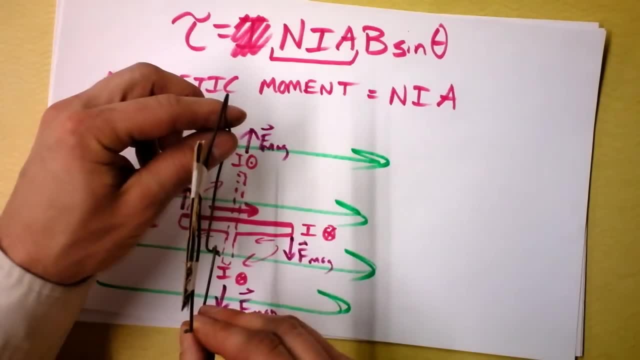 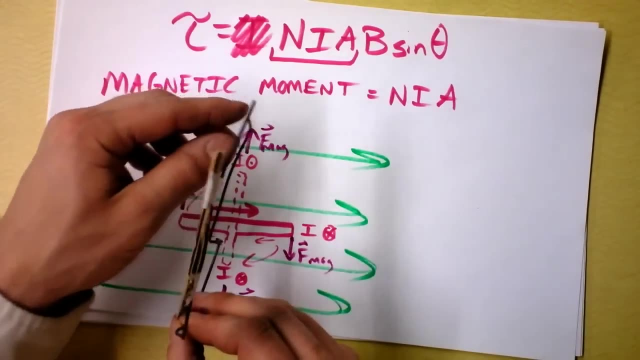 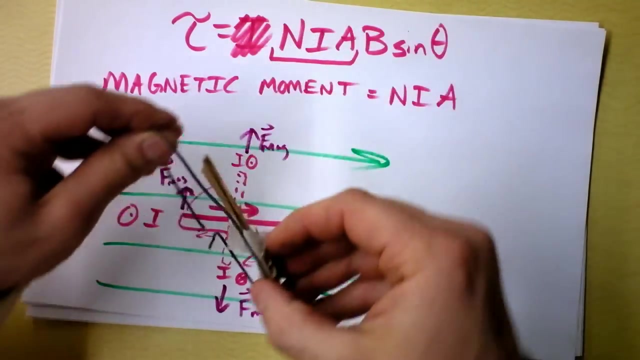 every time it makes it to this point right here. So instead of having a torque that brings it back, you have a torque that brings it to here and then switches the direction of the current like that, And then it'll go and faster.